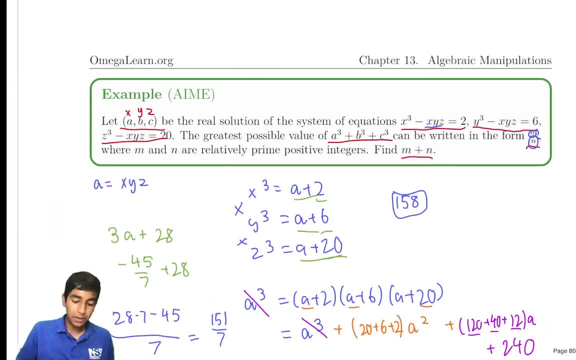 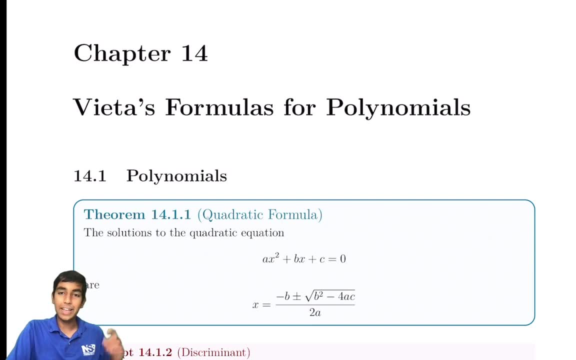 Last time, on Mastering AMC 1012,, we explored algebraic manipulations and how to solve complex looking equations using our techniques. Today we're taking a look at Viettas. Make sure to stay till the end of the video, where we'll explore how Viettas can make complex seeming problems. 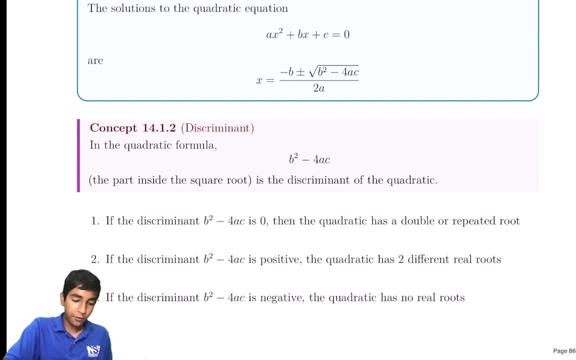 look like a piece of cake. Let's get started. So I'm sure you're familiar with the quadratic formula and how the discriminant determines how many real roots it has. So if it's zero, it has a double root. If it's positive, two real roots. Negative: there's no real roots. 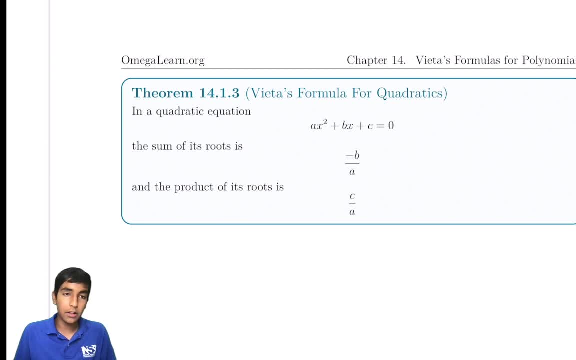 But what we're really here today is to discuss Viettas formulas, starting off with Viettas formulas for quadratics. In a quadratic the sum of roots is negative, b over a. the product is c over a. So if we have a quadratic like two x squared plus seven, x plus three equals, 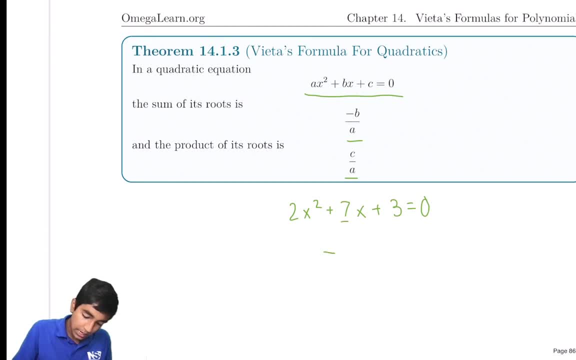 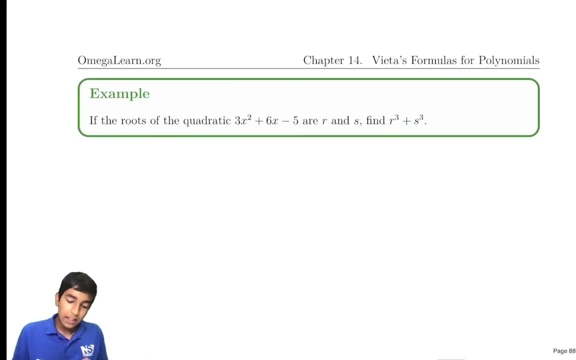 zero, the sum of roots is negative. of b over a, the product is just c over a, so three over a. Let's take a look at an example. but it's not just going to be a straightforward application. We're going to have to do a little bit of algebraic manipulation. 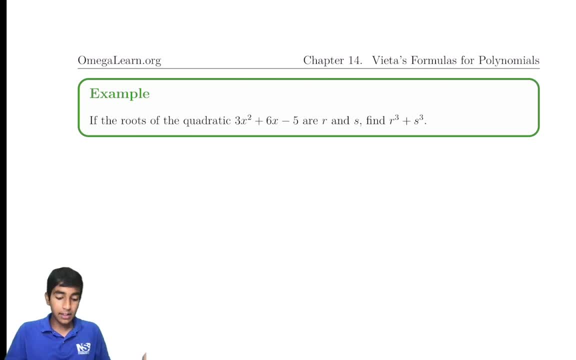 If the roots of the quadratic three x squared, plus six x minus five are r and s, find r cubed plus s cubed. How can we do this? We don't know. r cubed plus s cubed with Viettas. Let's figure. 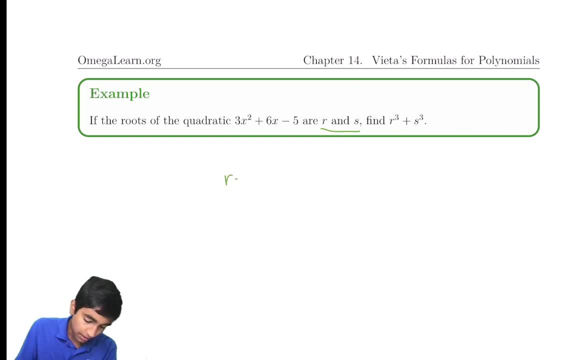 out what we do know with Viettas. We know r plus s. we know that r plus s equals negative of b over a. negative six over three is negative two and rs is just c over a, so negative five over three. But we're asked to find r cubed plus s cubed. 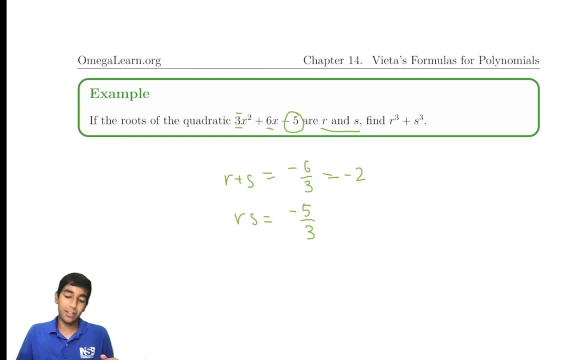 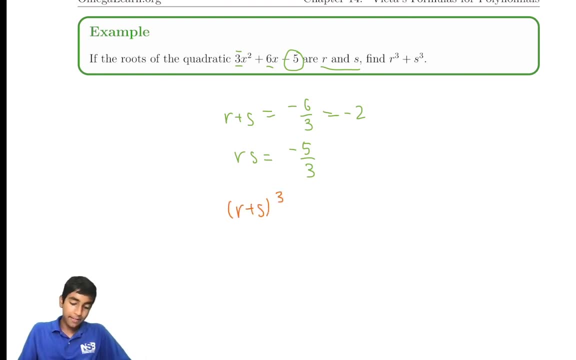 If you watch the factorizations video, you'll know exactly how to solve this. What we do is we cubed r plus s and this gives us r cubed plus three rs times r plus s, plus s cubed. This was one of the identities in the first video of algebra. 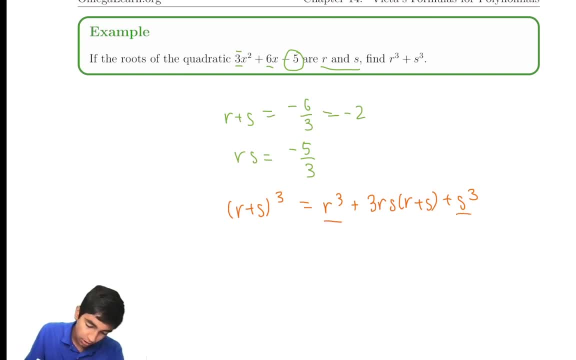 So we're asked to find r cubed plus s cubed. so let's plug in negative two. here We have negative two cubed equals r cubed plus s cubed plus 3 times rs is negative 5 thirds. so negative 5 thirds. 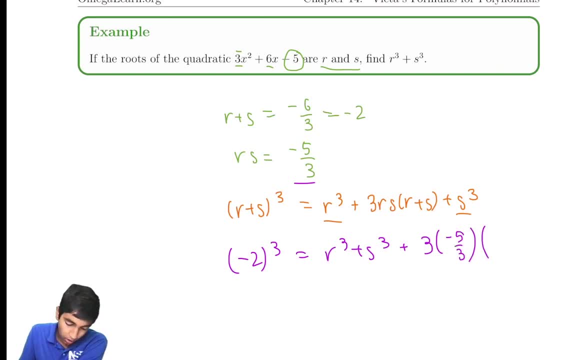 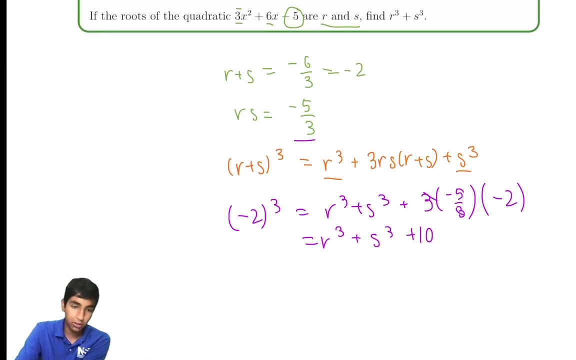 and then this is also times r plus s, which is negative, 2, 3's cancel and this is just r cubed plus s cubed plus 10. but we're asked to find, we need to find r cubed plus s cubed, so we just subtract 10 from both sides. 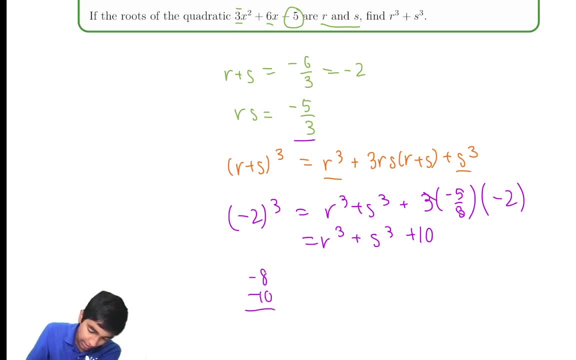 to get negative 8 minus 10 equals negative 18 as equals r cubed plus s cubed and negative 18 is our answer. so this problem kind of shows a standard Viettastric which is cubing, using algebraic manipulation sometimes, but in general it will all come down to these core values. 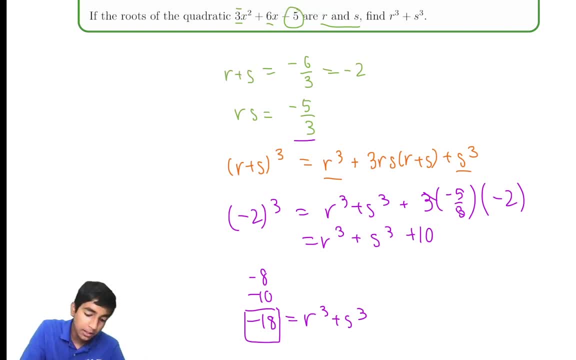 r plus s and rs. another thing you might see is to find 1 over r plus 1 over s and notice that this is just r over rs plus s over rs, because these terms will cancel to make 1 over r and these terms will cancel to make 1 over s. 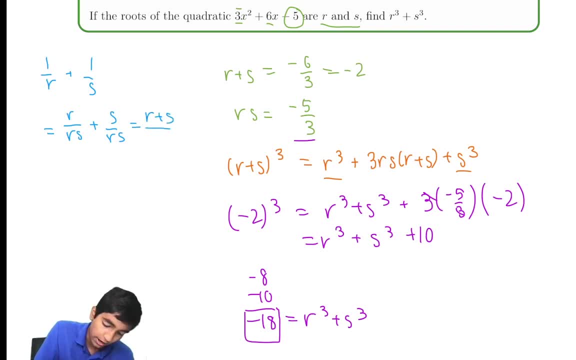 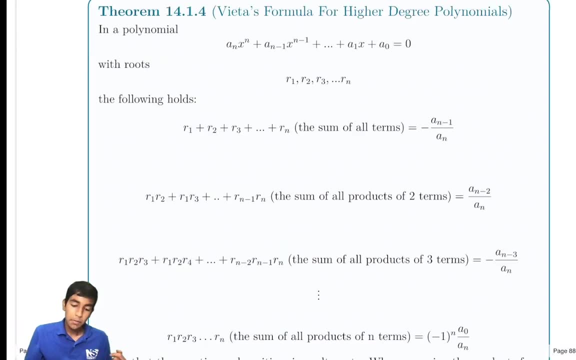 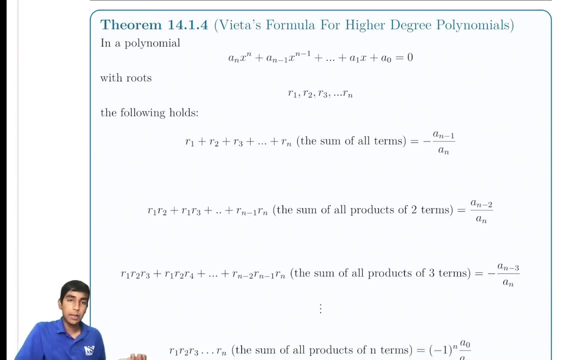 so this is just r plus s over rs. so you'll often have to do many manipulations to get what you're truly asked to find. but Viettastromalos isn't limited to quadratics, and no, it gets much more complex when we're dealing with higher degree problems. 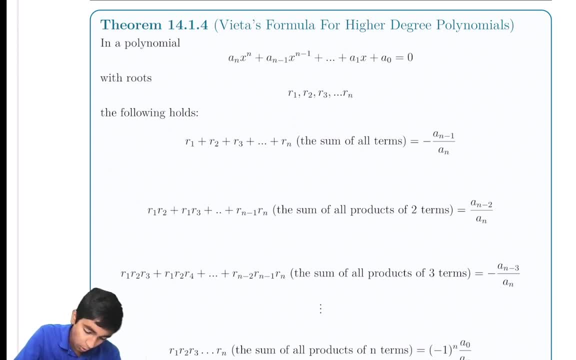 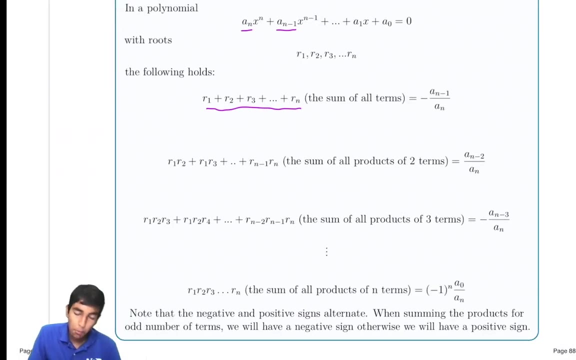 like polynomials, so in a polynomial of the form like this, we're asked to find what does Viettas tell us? it tells us that the sum of the terms r1 through rn is negative of this term, over this term, the sum of the products of two terms. 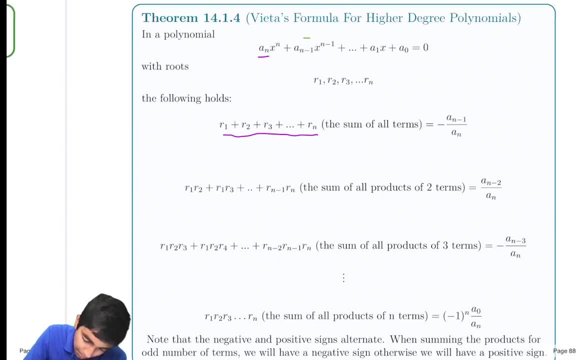 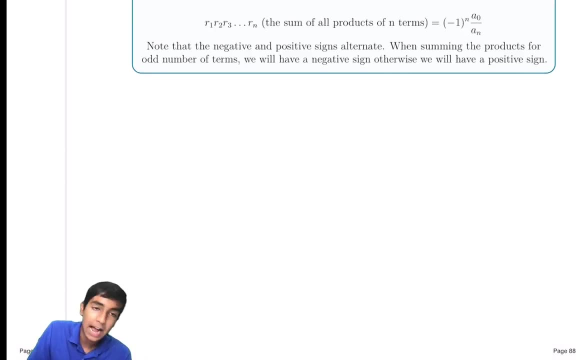 is the positive of of a n minus 2 times x to the n minus 2. now I know this seems scary, but let's see how this is used in an argument for an actual polynomial. let's say we have a polynomial x cubed minus 7x squared. 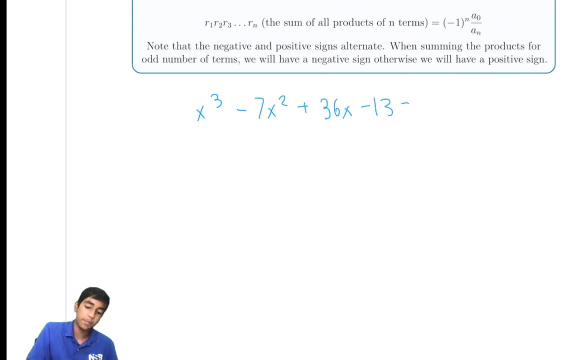 plus 36x minus 13 equals 0. the sum of the roots equals negative of negative 7 over the coefficient, which is just 1 in this case. and the reason we have? we have a negative here. now what we do is to get the sum of 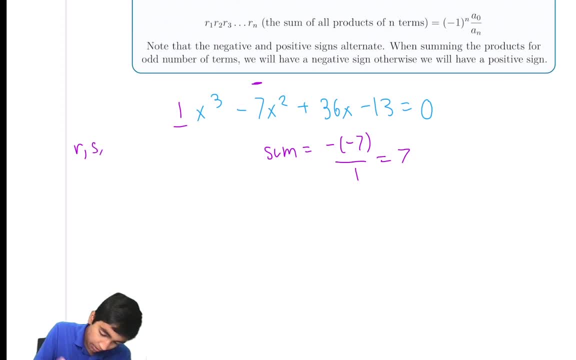 if the roots of this polynomial are r, s and t, then rs plus st plus rt, that would be equal to positive 36 over the coefficient, which is just 1 in this case. it's not always 1, just in this case, because it's just because it's a modding polynomial. 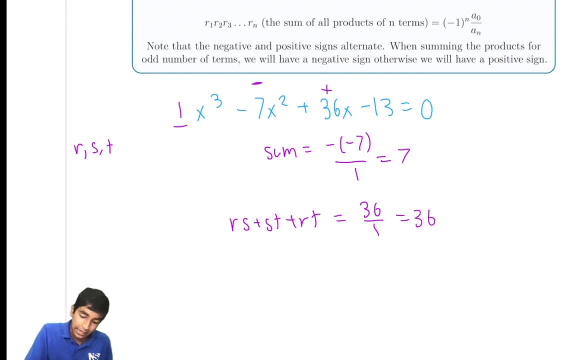 coefficient of 1 for x cubed, and then we go back to negative. so r times s times t is just negative of negative 13 over 1, which is 13. so the key here is that we always alternate, starting at negative, then positive, then negative. 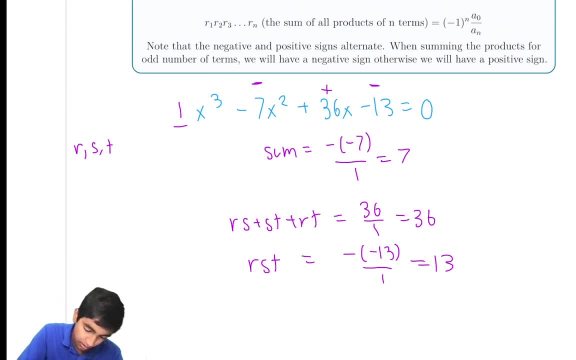 then positive and so on, and if it's helpful, you can write them out like this, like I just showed, and you can write out negative, positive on top of the coefficients. so then the sum of all the terms multiplied once, r plus s plus t, is just the first term. 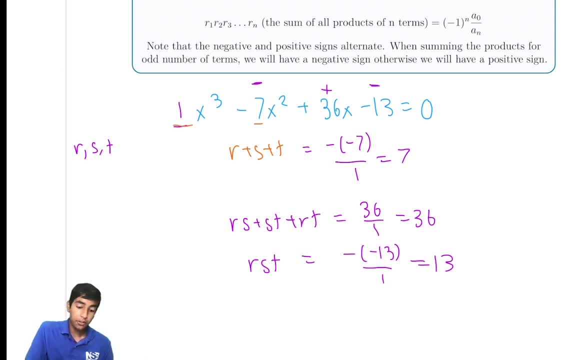 divided by the coefficient of the, the first term here that we the second term, I should say divided by the coefficient of the first term, times, whatever sign that's here- negative or positive or whatever- and next we have the sum of all the pairwise products, so the sum of all possible values. 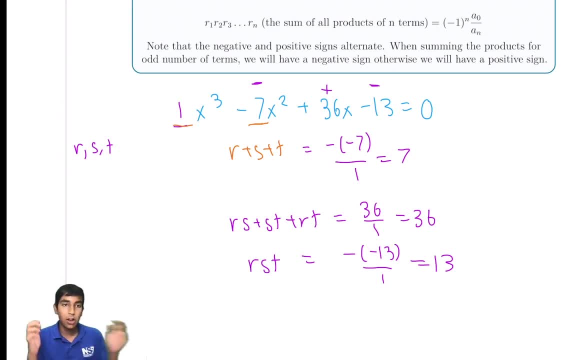 of the product of two roots, so rs, st, rt, that's going to be the second term divided by 1 over here. and finally, the sum of all products of three terms, so rst, that that will just be the third, the fourth term, the term here, divided by this term here. 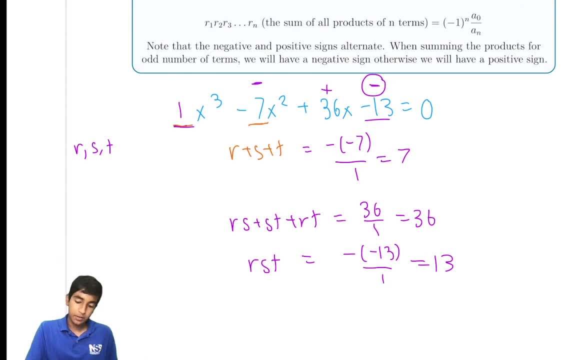 with whatever sign multiplied to five. let me take another example, just so you understand. this time we have x to the fourth minus seven, x cubed plus six, x squared minus thirty five, x plus two. let's find the sum of the roots. what we do is we label. 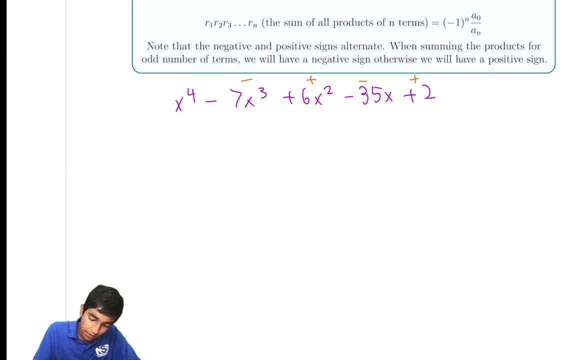 negative, positive, negative, positive, negative of negative seven, divided by the coefficient of one here, which is seven. so the sum of all four roots, let's say r plus x plus t plus u, this time is seven, and then, this time, the sum of all the pairwise products. now there's not just three sums. 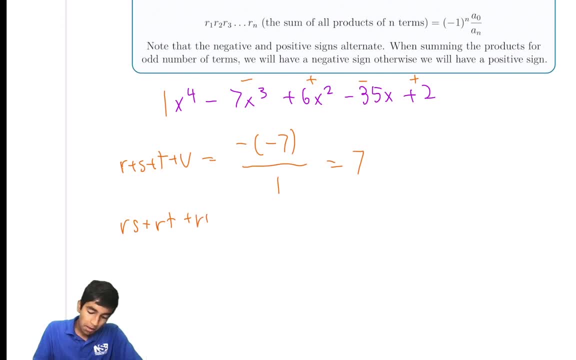 there's rs plus rt plus ru, plus st, plus su plus tu. the sum of all of those products, of all pairwise terms are attaches to one unit, that's just positive of six divided by one, the coefficient of x to the fourth, and then the sum of all three sums. 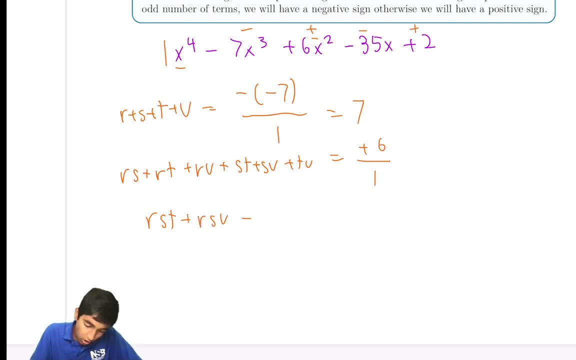 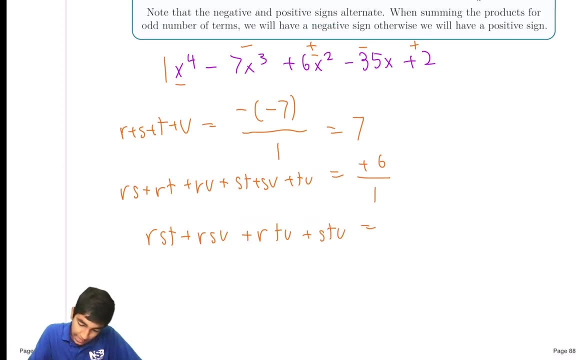 so rst plus rsu plus rtu plus stu is just negative, of negative thirty five, because that's the coefficient on this term divided by the coefficient on this term, which is one, 35.. And then the product, or the sum of all products, of four terms, but in this case 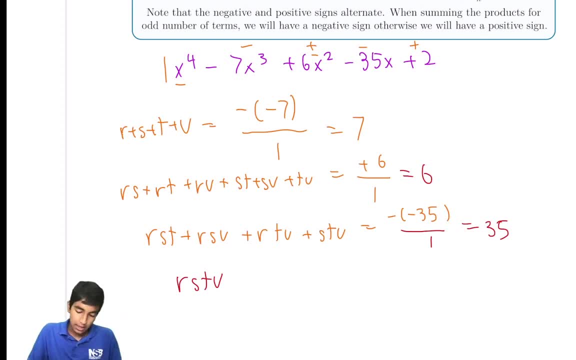 there's only one product for four terms. when we have four terms is positive. two over one equals two, And this first term does not always have to be one. It can be two or three, and we would divide by two, divide by two if that was a two instead. 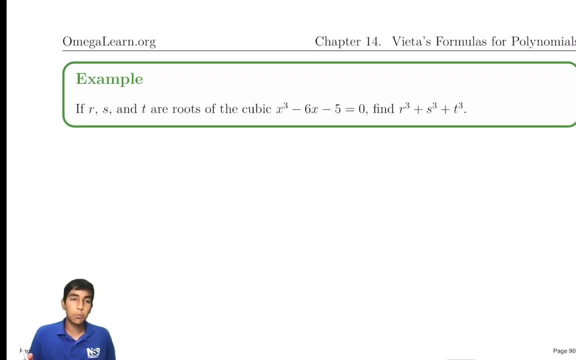 Now let's see how we can use this for an actual problem. If r, s and t are roots of the cubic, x cubed minus six, x minus five, find r cubed plus s cubed plus t cubed. What should we do here? 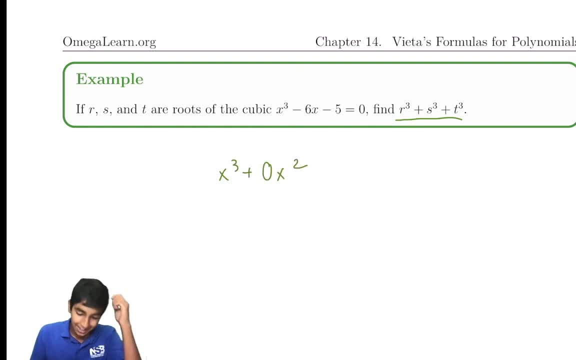 Well, first let's just write zero x squared, because the common mistake is to see that just read this as x squared minus six, x minus five, because there's no x squared term. Be careful, here you have a zero x squared, Always helpful. 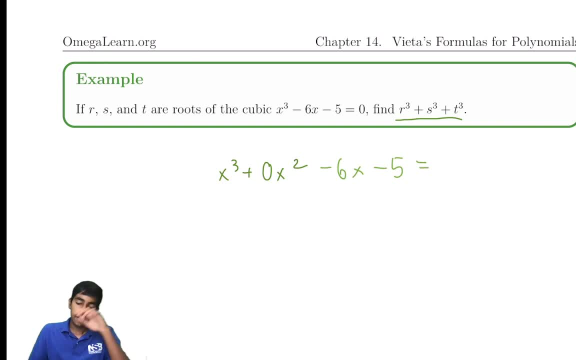 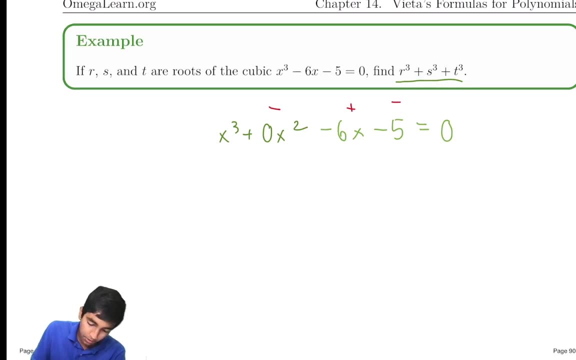 Write that out, You never know, Okay. so what does Viettas tell us? Let's write our standard: negative, positive, negative. So the sum of the roots r plus s plus t is negative of zero over one, which is just zero. 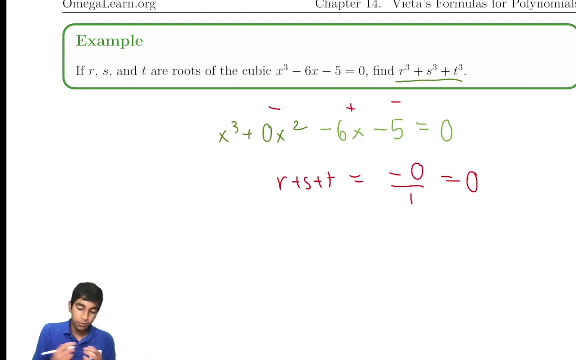 Now the sum of all the products of two numbers, two roots, rs plus rt plus st, equals positive of negative six over one. the coefficient here equals negative six. And then the product of the root rst is negative of negative five right. 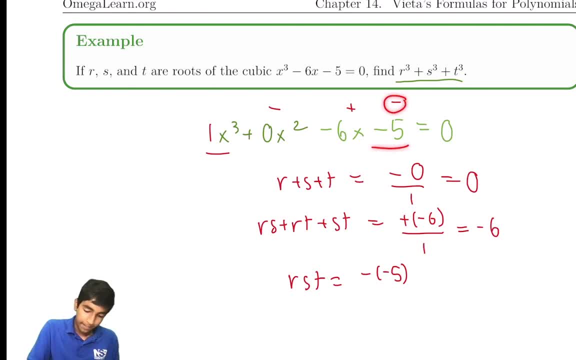 Negative sign of negative five over one, which is just five. But we're asked to find r cubed plus s cubed plus t cubed. What should we do? Do we know any identities? maybe, Again, if you've watched class one. 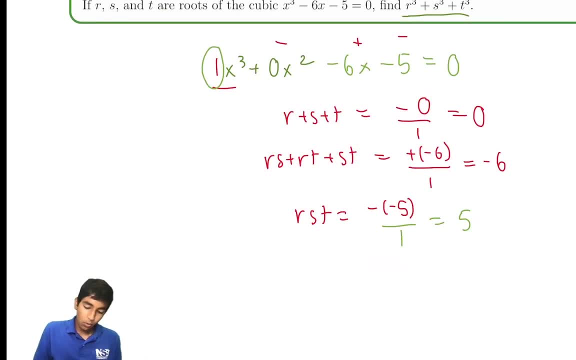 you should definitely watch the part one of the algebra series where you remember this identity. r cubed plus s. cubed plus t. cubed minus three rst equals r plus s plus t times. r squared plus s squared plus t. squared minus rs, minus rt, minus st. 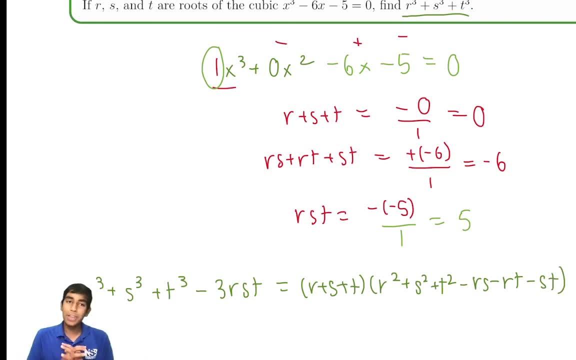 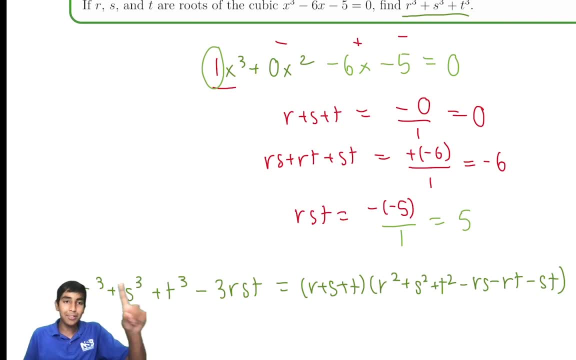 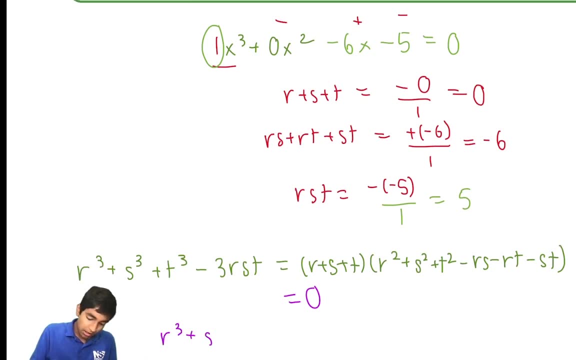 We don't even care about what that is. We already know r plus s plus t is zero. So this is just zero, And that means r cubed plus s cubed plus t cubed is nothing but three rst, which is 15.. 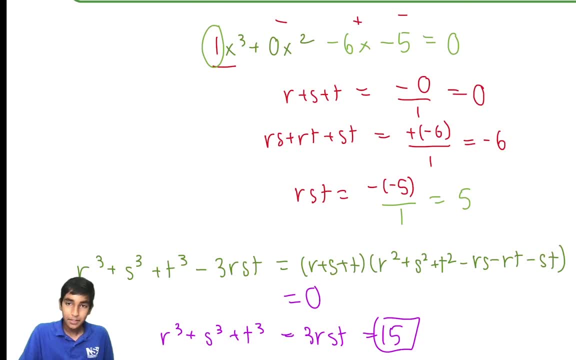 Isn't that cool. So the logic here was to see what does VS give us, And then always- not always, but often- you'll want to see what identities you can use. In this case, this identity saves us a lot of computation here. 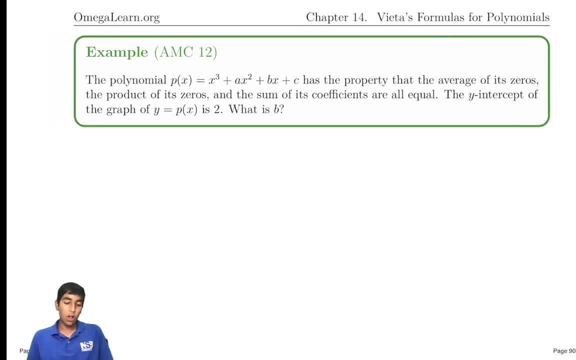 Okay, Now we're going to move on to a problem from the AMC12s. The polynomial a, cubed plus ax, squared plus bx plus c, has a property that the average of it zeroes, product of it zeroes and sum of coefficients are all equal. 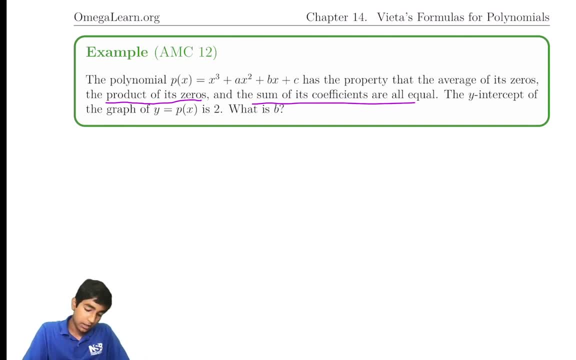 The y-intercept of the graph is two. What is b First? what does this last condition tell us? This last condition tells us that at x equals zero, p of x equals two, because the y-intercept is when x is zero. 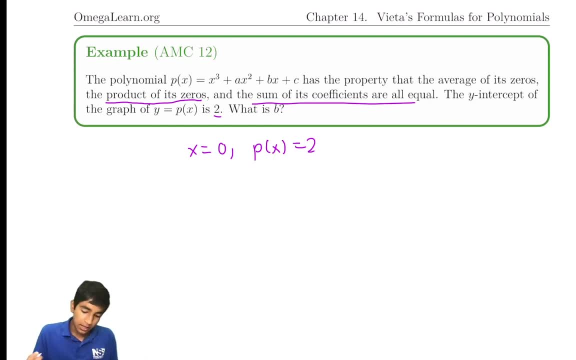 right in the center. What does this mean? What is p of x when x is zero? p of zero is just zero. cubed plus a times zero. squared plus zero, b plus c, This is all zero. So if this is equal to two, c is two. 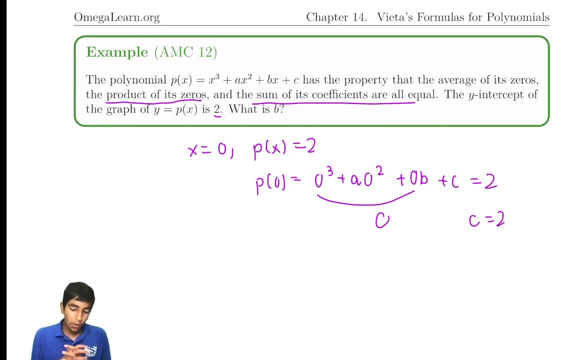 Okay, Now we're on to our VLs. What does VLs tell us? first of all, We know that the average of the zeroes, product and sum of coefficients are all equal. What is the average of the zeroes? There's three zeroes or roots. 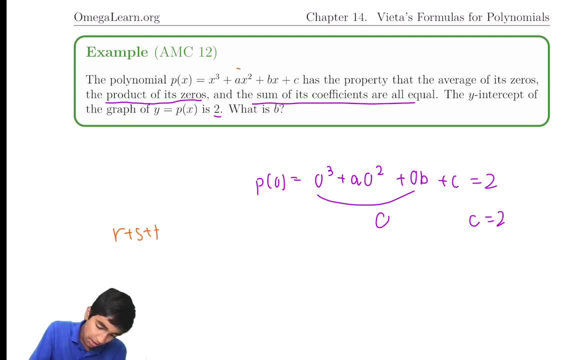 We know that r plus s plus t, let's write negative. positive. negative equals negative. a over one. the coefficient here? Okay, What about the product? But remember we're asking for the average, So it would be negative a by three. 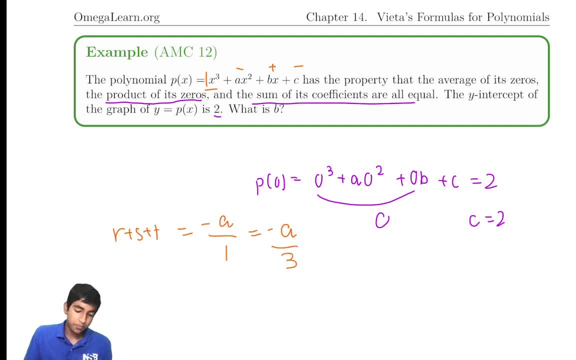 What about the product? The product is negative c by the coefficient here one. Don't forget this coefficient one here. I know it's one here and it doesn't really matter. but when the problem says two, then you'll be tricked. 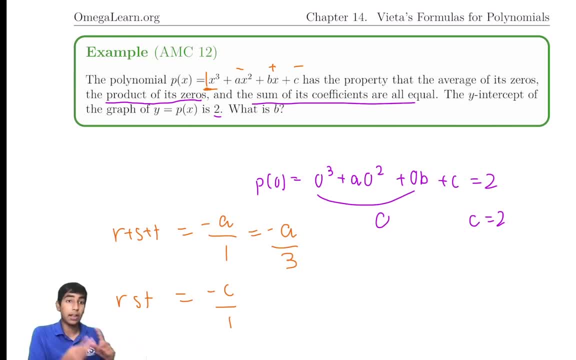 because then it's not just negative c. Okay, What about the product? Then it's not just negative c. So always be careful about that one term there. So negative c over one which is negative c. Oh, we know, it's the value of c. 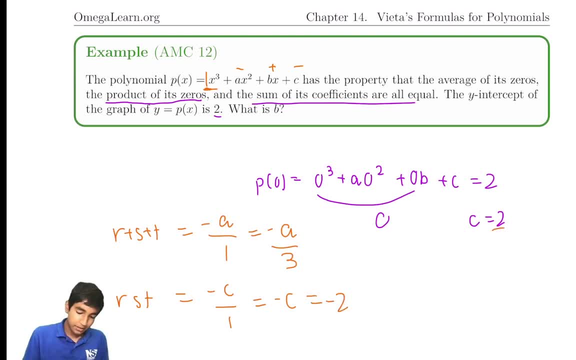 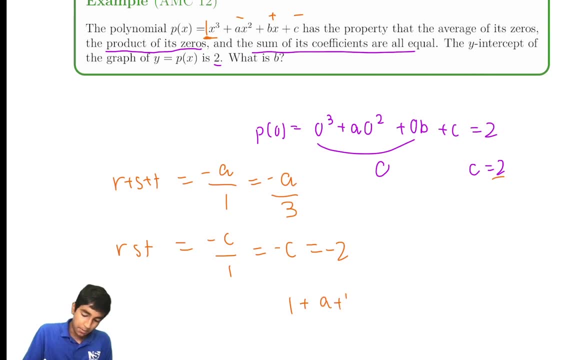 So this is just negative two. Now, sum of coefficients. The sum of coefficients is just one plus a plus b plus c, And we're given that this is also equal to both of these terms. First of all, we know, negative a over three equals negative two.